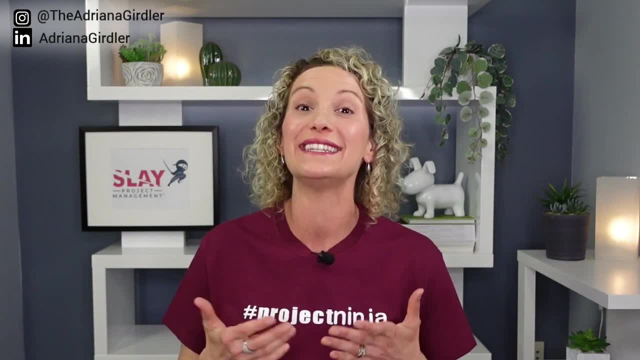 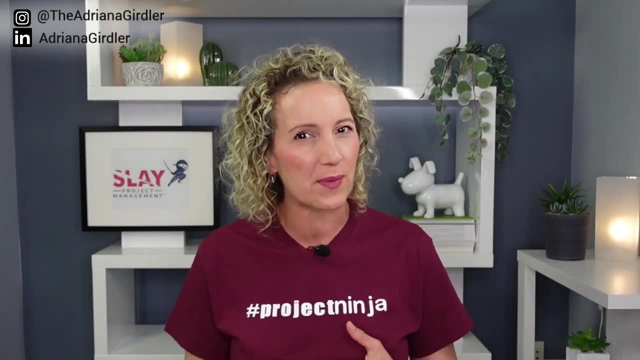 update report. it actually has some good information and it will be different than your last status update report, So that frequency is really important. Now, how would you distribute this? It really is dependent upon the type of document platform that you use. So if you're 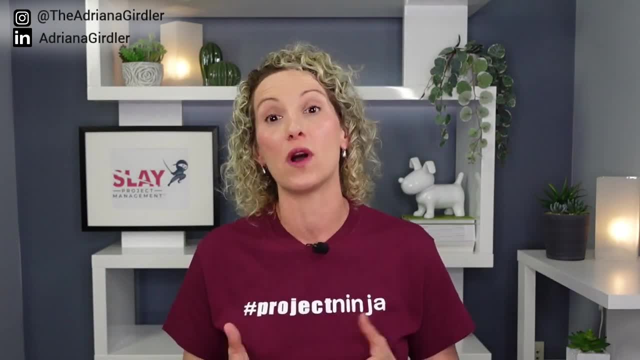 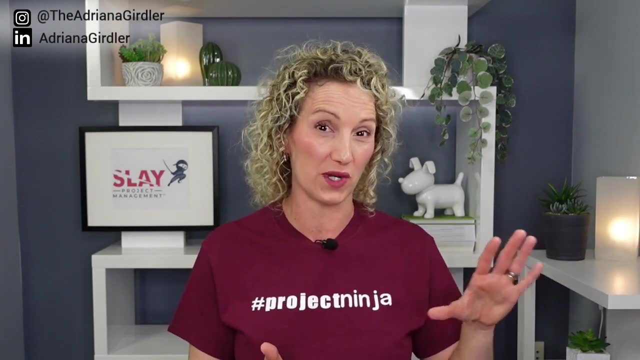 doing more of a Word document or PowerPoint. you may want to email that out to people and make that just a monthly reoccurrence. You may have a project shared drive that maybe you want to put it on there and people go to it. Or, like I said, you may want to use a web-based platform. 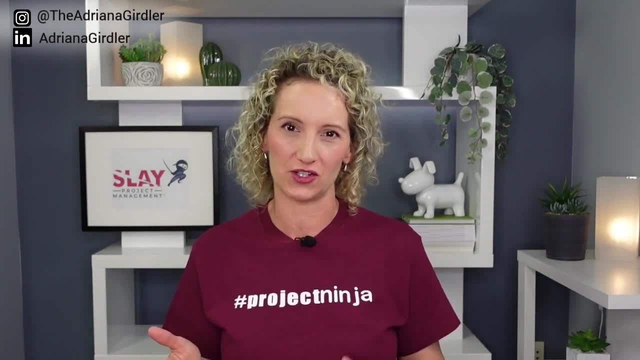 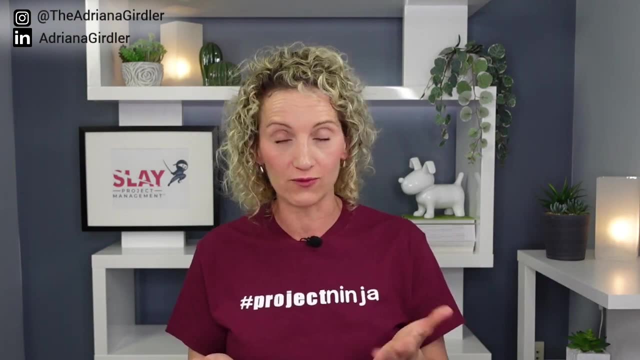 I use Microsoft Office SharePoint and I actually create all my project documents. So I'm there and I bring people to it. So there's definitely different ways depending on really how do you use and communicate with your projects. Now, what I'm going to show you next is what 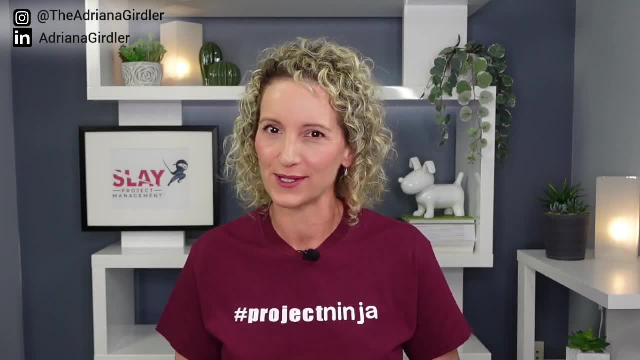 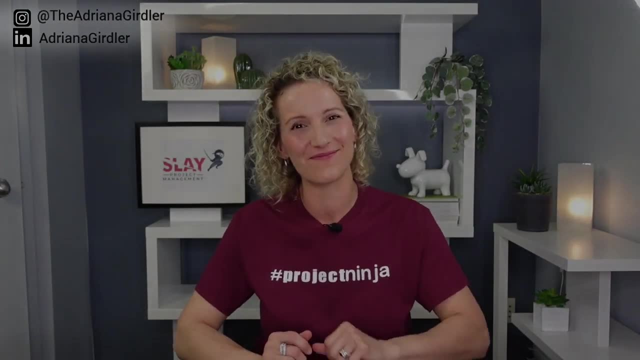 actually goes into that. status update report. Project summary. This is the first thing that you need to do, So let me show you an example. Follow me. So with here we have the title of our update, and it's a monthly update, And here's the date of it being updated. 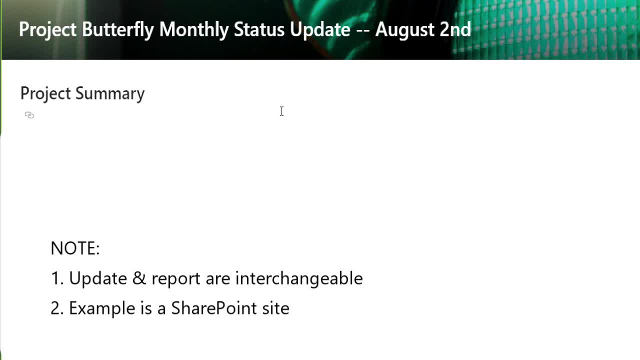 Which was the second and your first section. always in any update is a project summary. Now, there's really good reason for this. It's because you want to include information, to remind people, all those stakeholders, what it is that we're doing and what is it that you would include. 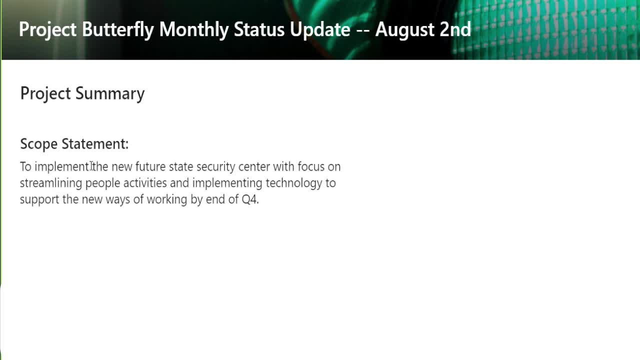 in this project summary? Well, the scope statement, which is: what is it that I'm responsible for from a delivery standpoint and for this particular project? we're implementing a new future state security center And it's very specific. You're going to want to make sure that there are no. 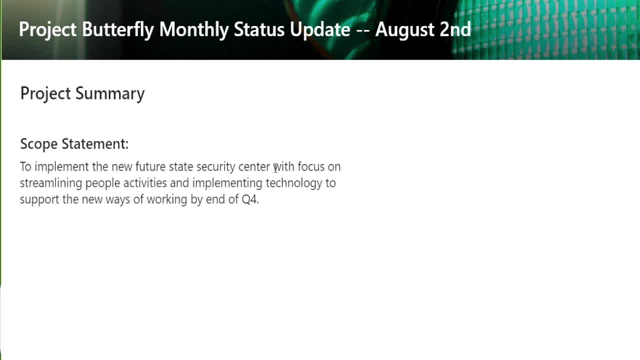 with focus on streamlining people activities and implementing some technology to support new ways of working. now we also include the project priority matrix because this is going to let people know what your constraints are, what you're willing to optimize and accept from a scope, time and budget. 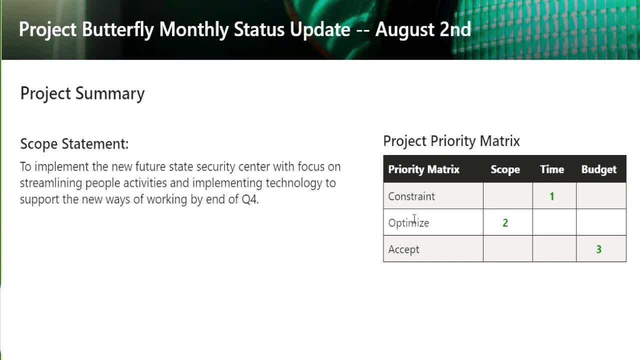 perspective. this becomes really handy when you have people off to the side asking you to, oh, just add this element without having an understanding of everything else, so you can bring them back to this and saying, hey, I can't do it. my biggest constraint is time, and what you're asking me to do is to 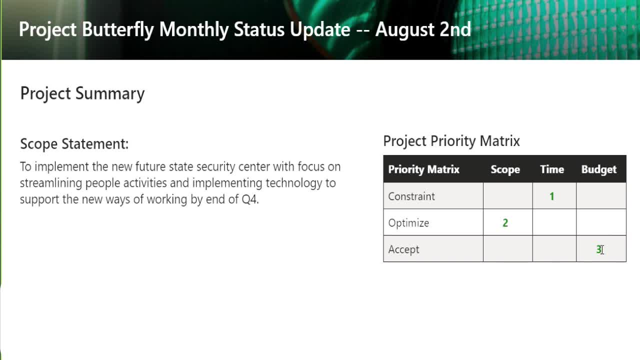 increase time unless you have money, which is budget- in order to help me out. I'm not able to do it, so it becomes a real powerful tool for you and, in fact, in my slave project management course. with the link under this video, I actually go into this in great detail. I love this project priority matrix and 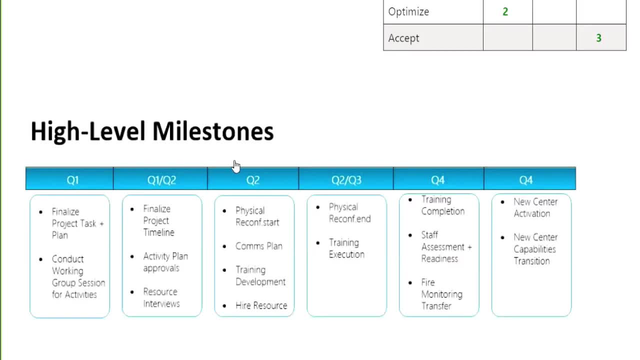 now, the next thing that you would have in your project summary is your high level milestones. not your detail, just very high level. you want to give an overarching view to anybody who's looking at this. what is it that we're doing and when are we delivering it by? it's really very 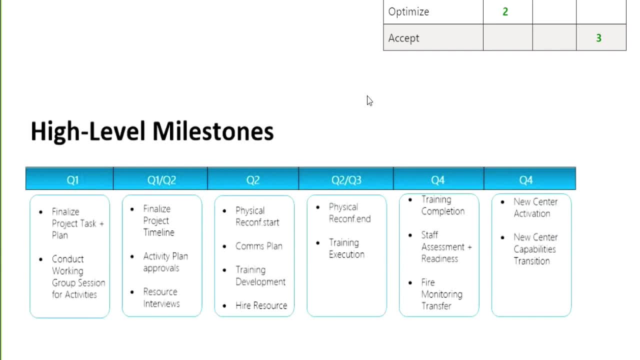 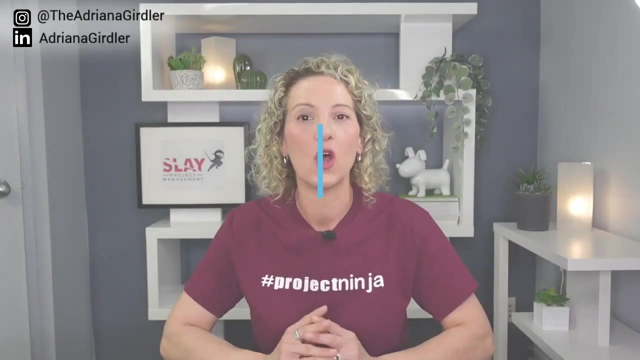 high-level. it supports a scope statement in the priority matrix so that anyone coming into it, especially a brand new person, can get very quickly what is your project all about? so when they read the rest of the information in your status update, it makes sense overall project status. so this is very 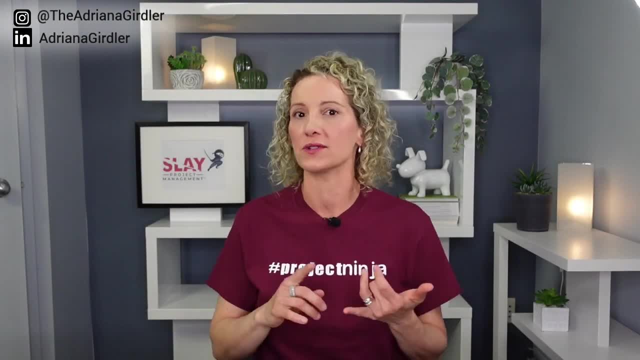 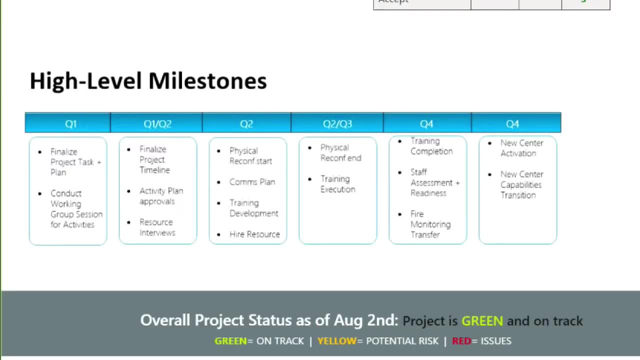 simply put: what is the overall status of your project? are you on track or at risk? let's go back to that example so I can show you more. okay, now we want to go to the overall oops project status, which is basically saying, overall, my project as a 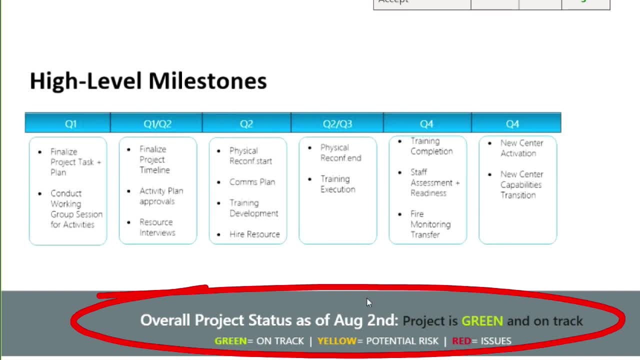 whole. how is it? is it on track? do I have some issues? I like to use a stoplight system of green, yellow and red, and green just means you're on track. yellow: I may have some potential risks, but we're working on it. in red is I definitely. 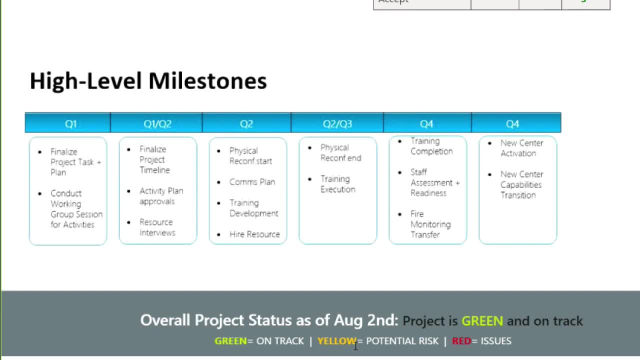 have some issues. I'm probably going to need some intervention in order to ensure that I get out of that. not a bad thing to have any reds or yellows. in fact, I always tell everyone: you need to have reds and yellows. if I come across a. 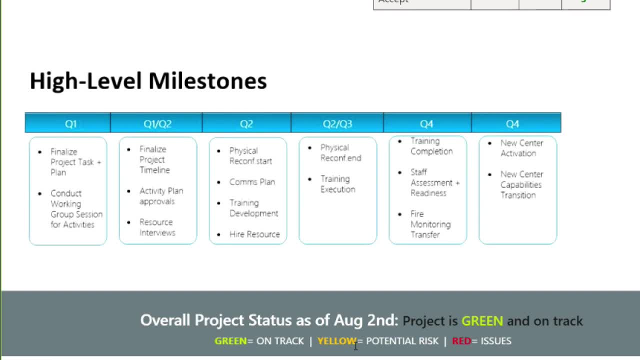 project that's always in green status. I question it and saying I don't know if they actually know what's going on, because I've never come across a project that is constantly 100% in green strut status on track, unless it's just myself and I've complete 100% control. so if someone were to just look, 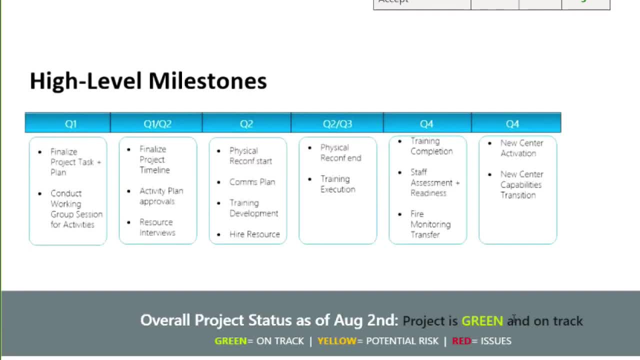 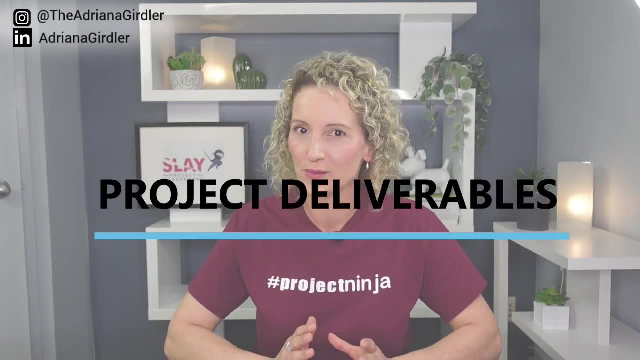 quickly and look at the right way to navigate across the green screen is the at the project summary and they just want to say, hey, how's this project? Right away, immediately they know this project overall is on track, Project deliverables or major milestone status. This is the heartbeat of your status report. 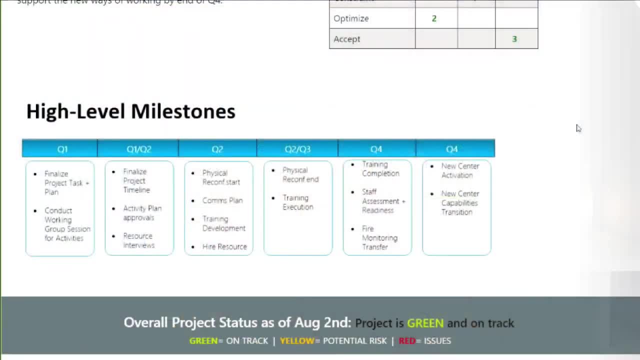 So this is where all the detail is going to be. Now that we have the project summary, which is really important, we have our overall status, which I'm saying is green. Now we're going to get to the heart of this project status update, and that is project. 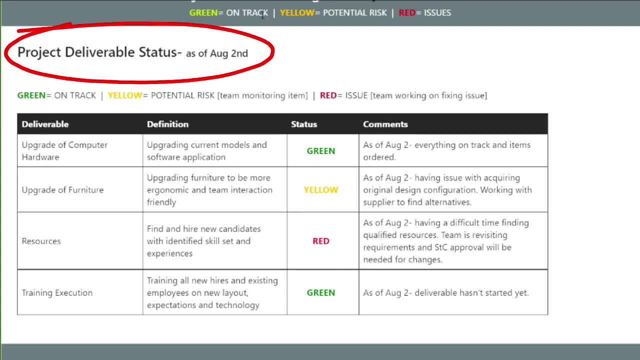 deliverable status. So, again using the same stoplight system of green, yellow and red, I'm now going to be very specific to what deliverables I'm going to be giving a status on. Now, what I usually do is in my charter. I know what my major deliverables are. 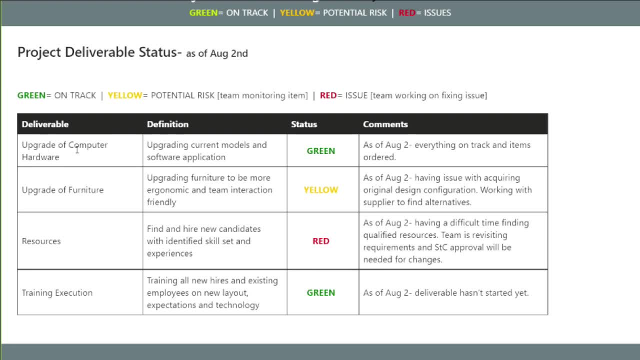 and I'm just going to use those same deliverables in my monthly status update, So this is not an exhaustive list. This is just an example I'm giving you in regards. This was an actual, real project and, due to confidentiality, I can't necessarily put everything in there. 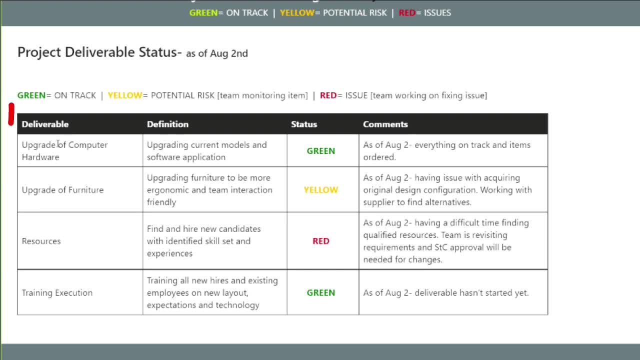 but just to give you an idea of some things. So, from a deliverable standpoint of this project, we had upgrade of computer hardware, upgrade of furniture, We had to look at hiring new resources and we had to do some training. Believe me, there's a lot more, but for this example, 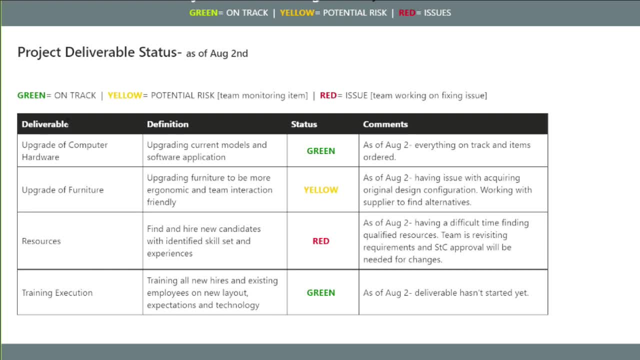 I just want to make it short and sweet for you. Now. it's really important, because this is the heartbeat of everything. This is where you're getting the nitty gritty is define what your deliverable is, because I promise you, people come in with assumptions. 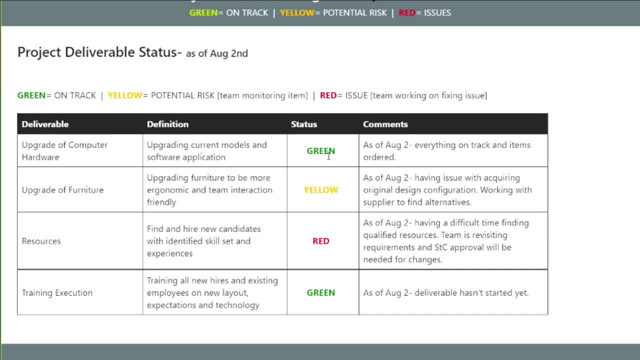 and you want to negate those assumptions by just defining it. And then you want to give your status for each one: green, yellow, red, green. Again, do not be afraid of having reds and yellows. It just means that you understand your project. You're on top of everything. 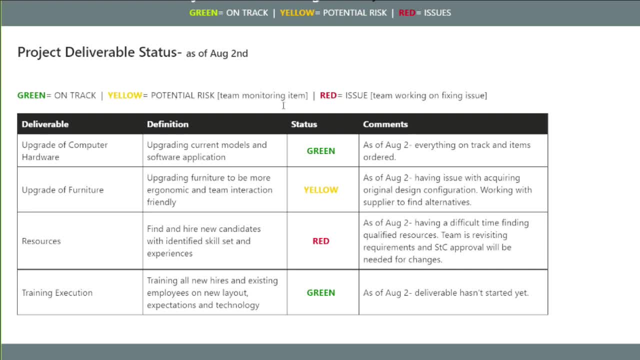 And don't forget here: yellow potential risk. but the team is monitoring them And if I have a red it means my team is working on fixing the issue. That could be literally them going in and doing it themselves, me reaching out to maybe some steering committee members. whatever it may be. 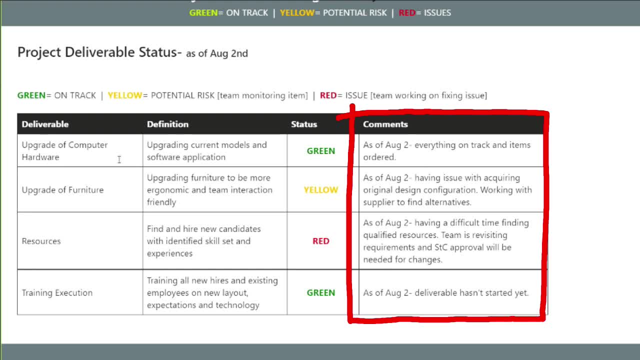 And your comment is for each deliverable. So, for example, the upgrading of the computer hardware. As of this update, everything's on track. Items have been ordered. Great, Updating, upgrading our furniture. Well, we're having some issues because the original design configuration. 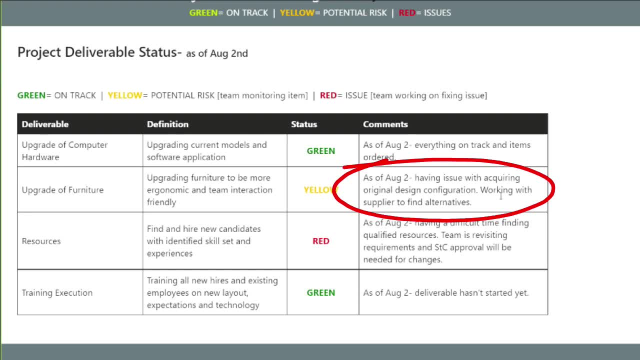 we can't seem to get what we originally thought we designed and we're ordering. So we're trying to find alternatives with ourselves. So we're going to go to our supplier. That to me, is a yellow. We're monitoring it, We're coming up with an alternative solution. It's not a red because it's not an issue. 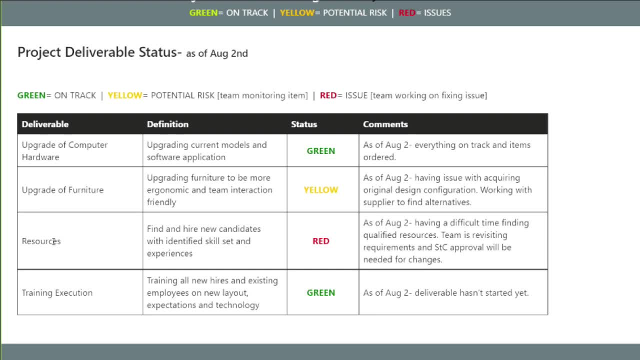 It just means we have to find a different solution for it. Resources I marked down as a red because we're having a difficult time finding qualified resources. We're going to revisit our requirements and definitely go to our steering committee to get approval for those changes. 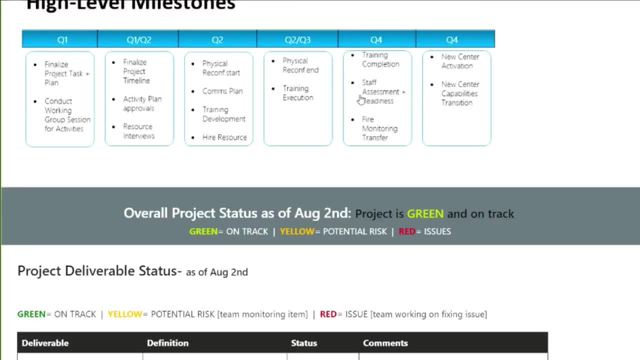 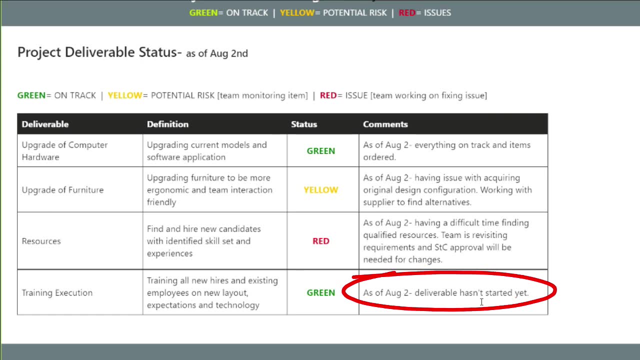 And then I got some training, execution, which if I were to scroll here, it's really towards the end of my project And I'm not there yet. I just said, as of August 2nd, Deliverable hasn't started yet, So I'm giving myself a little bit of a bonus by saying it's green. 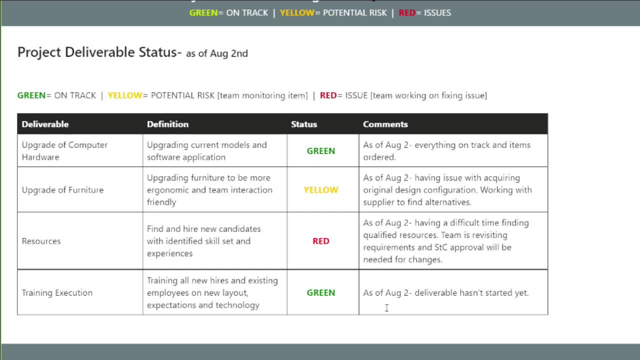 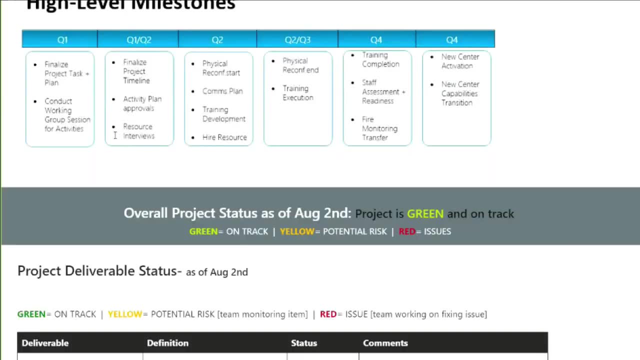 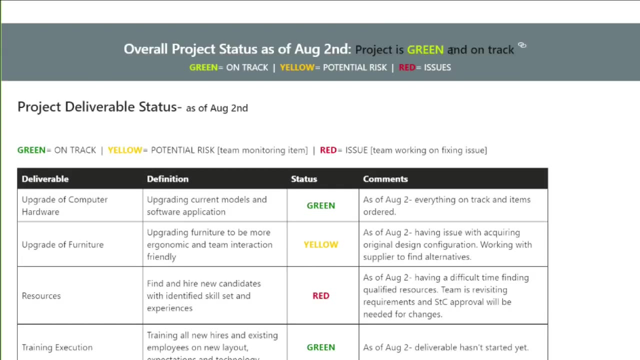 It's on track. because it is on track, I'm doing everything else in order to make it work. So this is your heartbeat. Again, you want to have your project summary so that people understand it And even though my project Deliverable has some reds and yellows, I still feel as a project manager. my project is green. 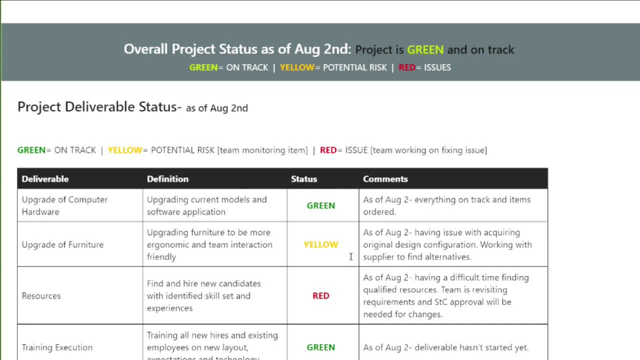 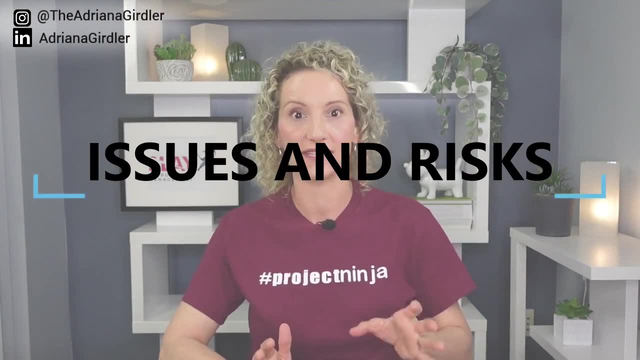 Even though I have a few yellows and reds, because I have plans in place in order to address them. Issues and risk: This is where you're going to outline some high level external elements that are impacting your project that you want to share with your stakeholders. 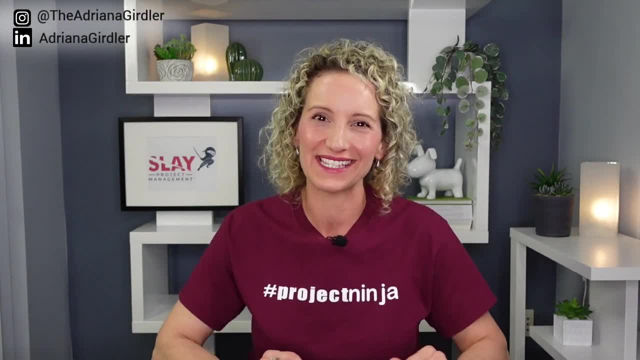 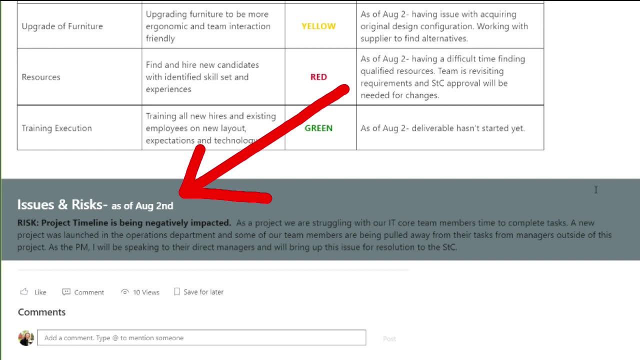 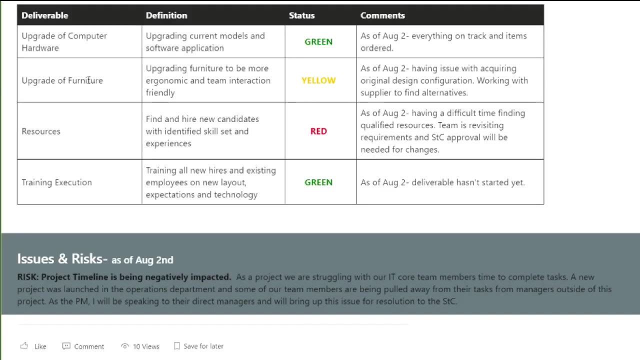 Anything that's going to impact scope, time or budget. Let's go back to that example. Now we're going to go to the last section of your status update: issues and risks. So this is where you're going to highlight any issues that are not connected to a Deliverable, because there are things like that. 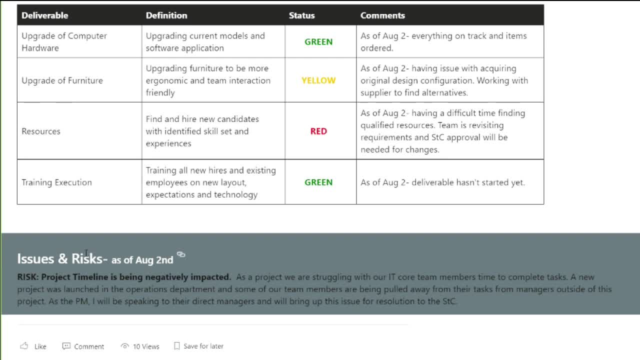 And you just want to give some information and any risks that you are identifying. you want to place it here Again. you want to show your due diligence, that you know what's going on with the project and anything that's going to impact your scope, time and budget. 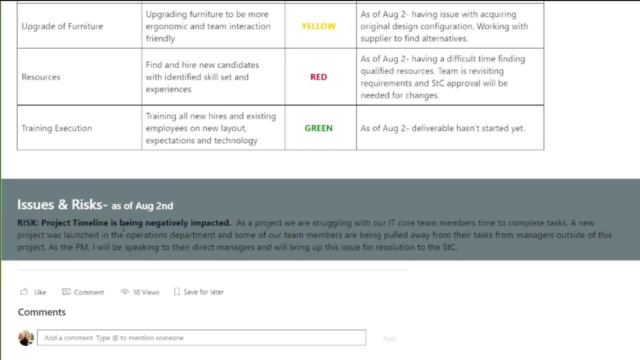 So with this section, I actually have a risk, and that's project timeline is being negatively impacted. And now this is where you give that information. What is it, How are you going to address it And is there anything else of note? So why? 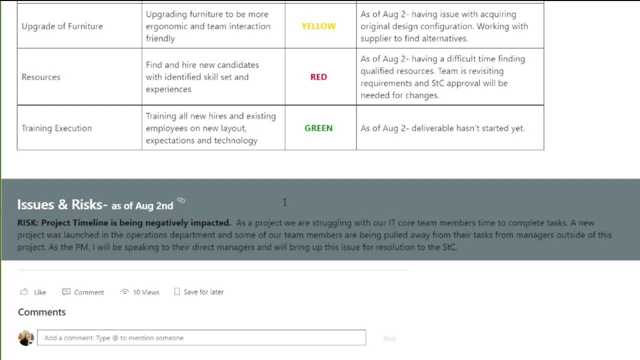 Why is it important? Why is my timeline being negatively impacted? is because, as a project, we're struggling with our IT core team members to complete their tasks in the timeline associated. We all have had that issue, but this is not about finger pointing. 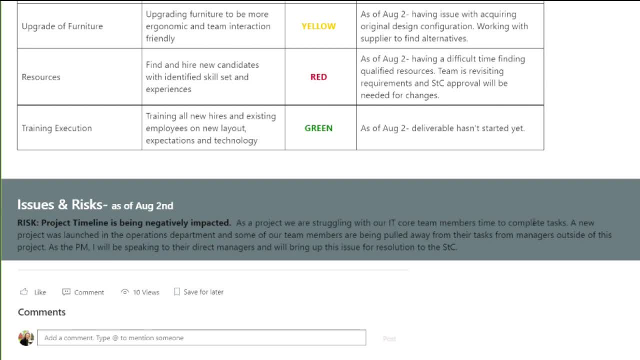 I'm now even going into greater detail. Why is this happening? It's not because they don't care. They do care. It's a new project was launched. And what happens when something new happens? It's new, it's shiny, it's exciting and everyone is told to start working on it. 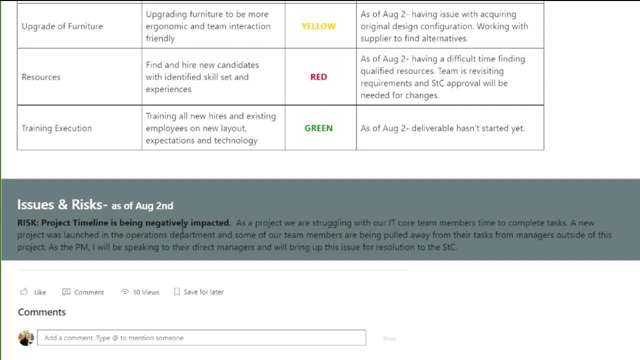 But now they're actually The department that launched this new project. they're pulling my team members away from me. Why? Because I don't have a dedicated team 100% to this project. In fact, they have a whole bunch of other projects, my subject matter experts. 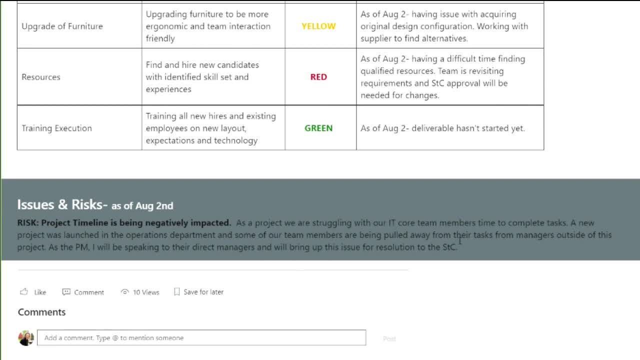 So it's a balancing act, But I'm now calling out saying that their managers are pulling on them to say, hey, start working on this project. So it's now my job. What I'm going to do as a PM is to speak to their direct managers. 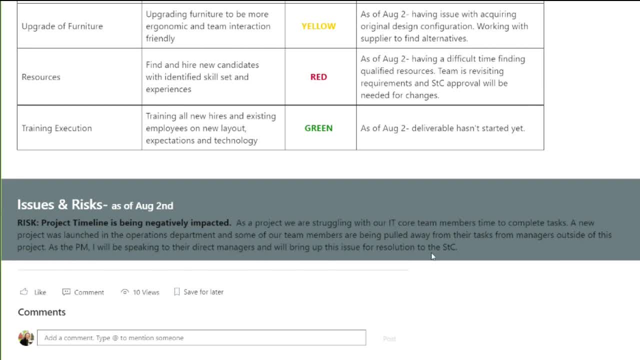 I'm going to bring up this issue for resolution to the steering committee because that's their job- To remove my roadblocks. So I just have to make sure that there's a balance of time for my team. Am I worried about this risk at the present moment? 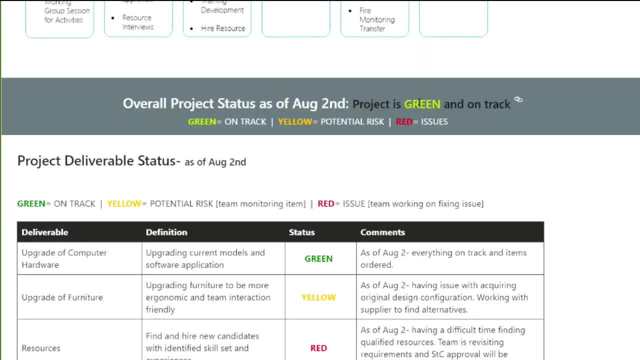 Not really. That's why I said green. But if I start talking to direct managers and steering committee and nothing happens, then my project is going to go into the red very quickly. But I'm going to at least show my due diligence and I'm going to show the paper trail that shows that I told everybody this. 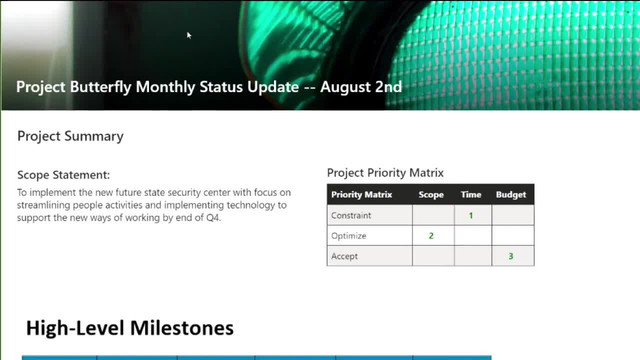 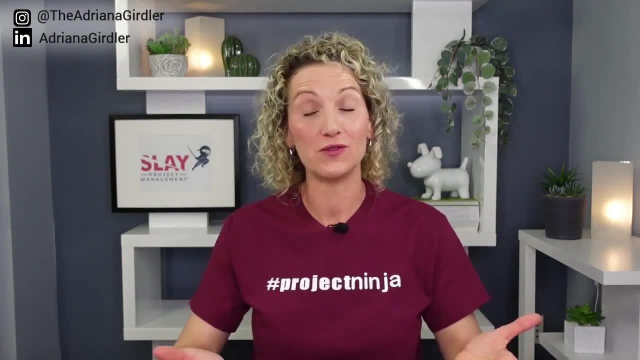 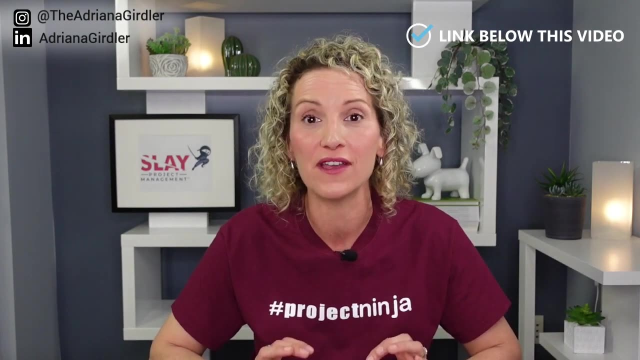 Again, this update is powerful And I highly recommend that All your projects have one. Now that you know how to create a project status report, it's now time for you to go to the link under this video and grab your seat for my free training on the Fab Five Fundamentals of Project Management. 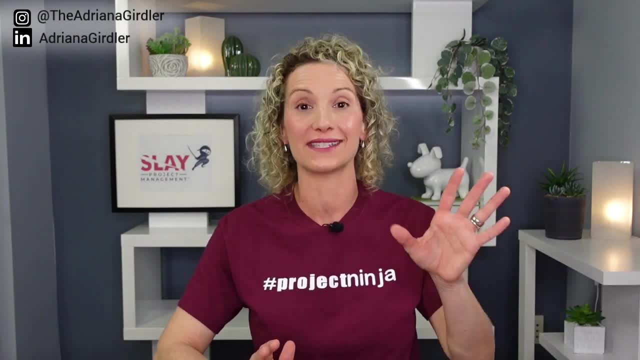 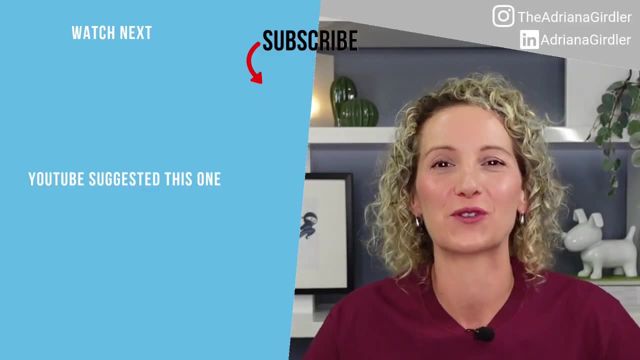 If you're here for status reports, I'm letting you know: go there, because it's going to give you some really key elements are just going to help you be amazing at project management. Don't forget to subscribe to the channel, like this video and please share it with all the people. 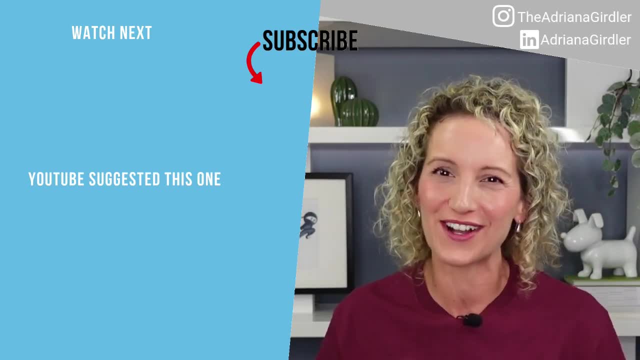 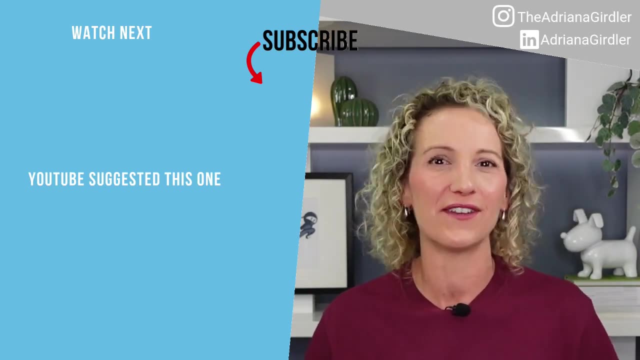 You know it really helps us grow our community, giving you more great content. I really hope you like this video and please let me know if you have anything else that you would add to this. Any comments you have, please put them in the comments below. Until the next video. See you later. 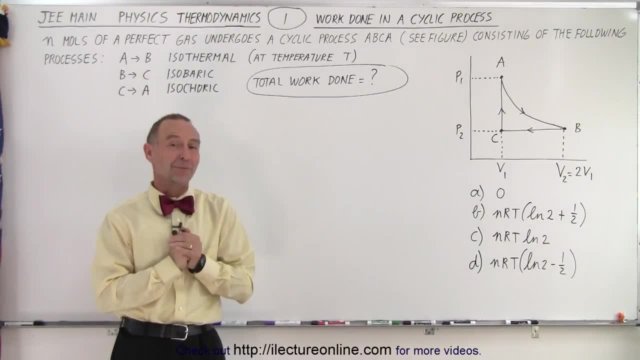 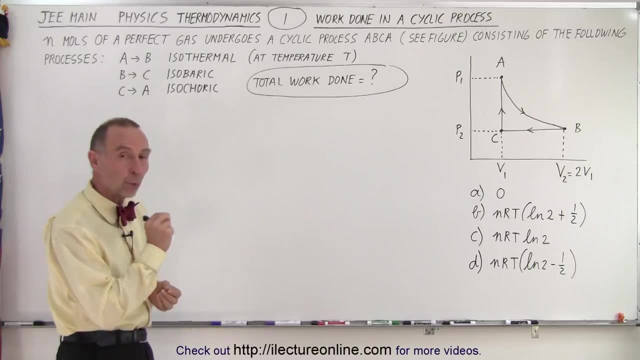 Welcome to our lecture online. Here's a really interesting problem. I actually like a problem like this- and it deals with a cyclic process and they're asking us to calculate the work done in a particular cyclic process. So let's read the problem: Cyclic process. Okay, let's call it. 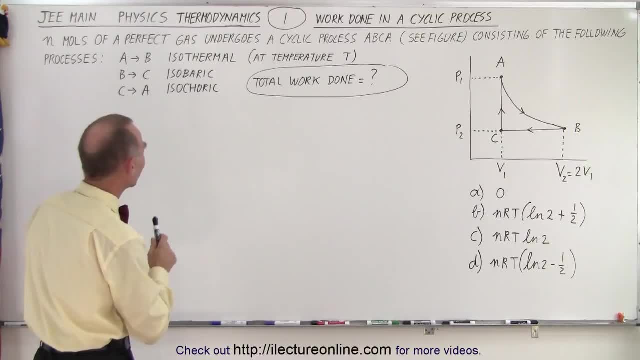 a cyclic process. N moles of a perfect gas undergoes a cyclic process from A to B to C and back to A. see the figure consisting of the following processes. So, from A to B, we have an isothermal process, Thermal or isotermic, Hmm. well, from B to C, we have an isobaric process. 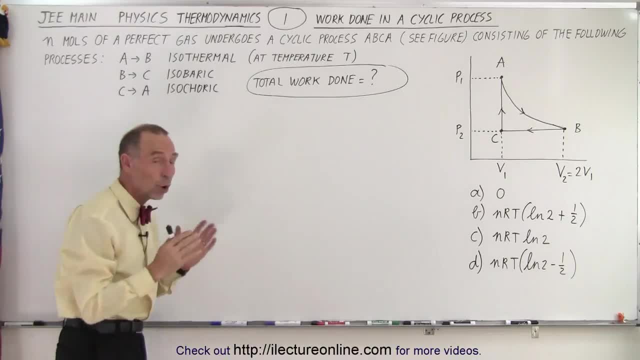 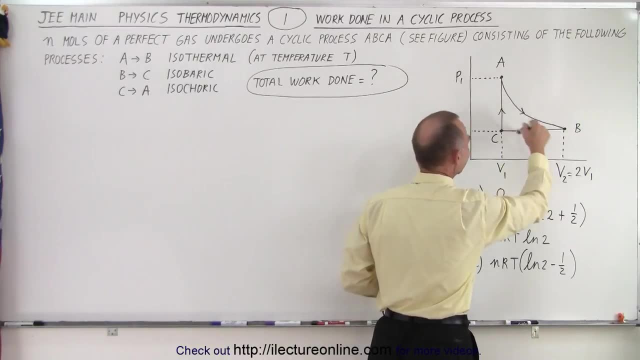 from C to A. we have an isochoric process and they're wanting to know the total work done. So typically the work done equals the area inside the cyclic process, but since one of the curves is along the cyclic process, it says there's no cyclic process inside the cyclic process. 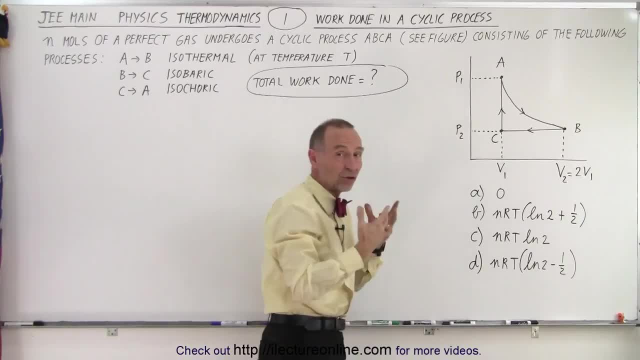 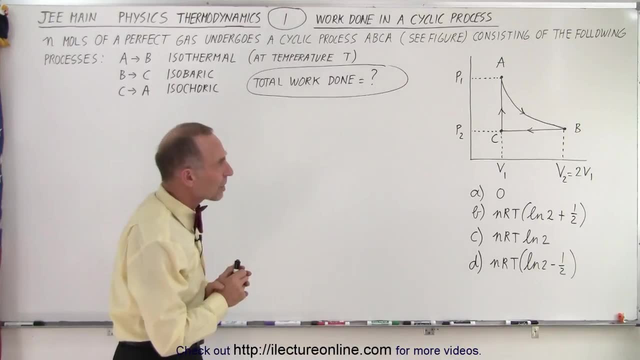 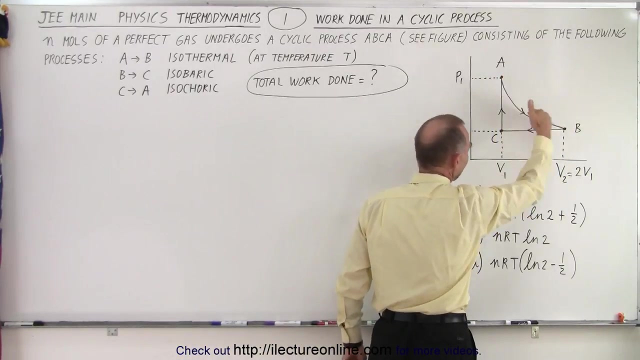 logarithmic curve. it's not easy to calculate it simply by the geometry. If this was a straight line it would be easy, but it's an isothermal process. So what we need to do here is we need to figure out where work is done. Now, going from A to B, work is done by the gas, so that's called 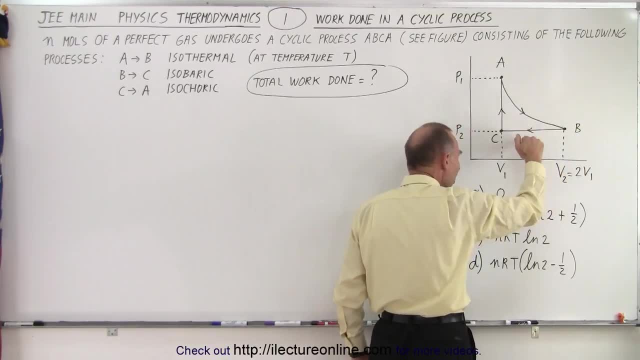 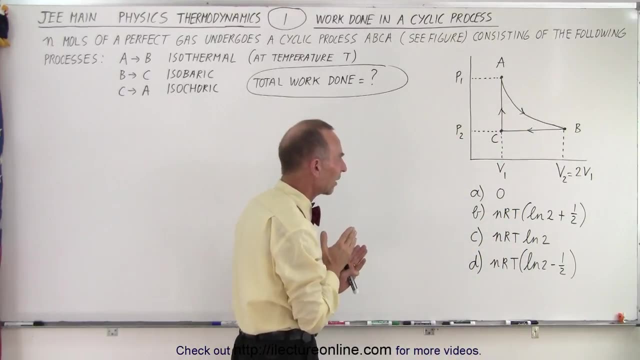 positive work. Going from B to C, work is done on the gas, that's negative work. And then going from C to A, no work is done because there's no change in the volume of the gas. You can only do work if 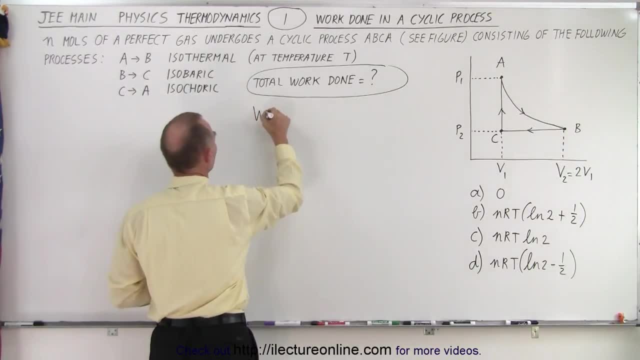 there's a change in volume. So that means that the total work is equal to the work done from going from A to B and then plus the work done going from B to C. but that's going to be a negative quantity because we're compressing the gas and if you take the definition that it's work done by.